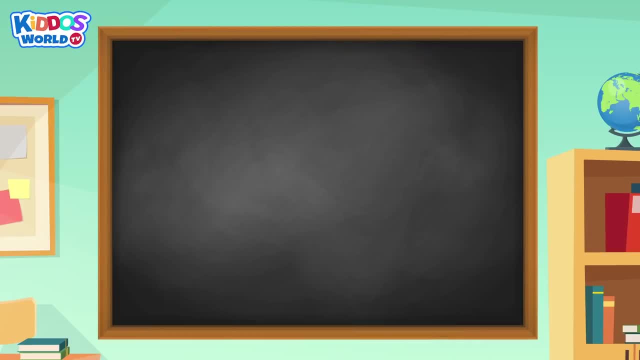 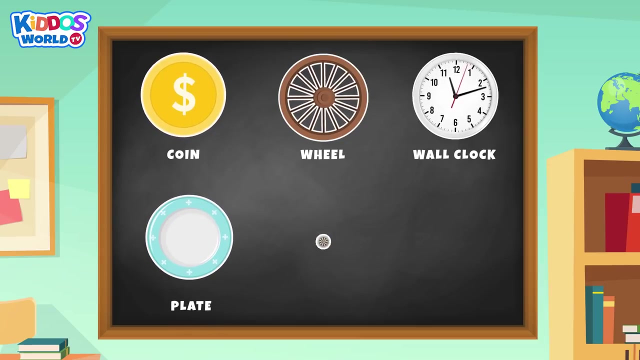 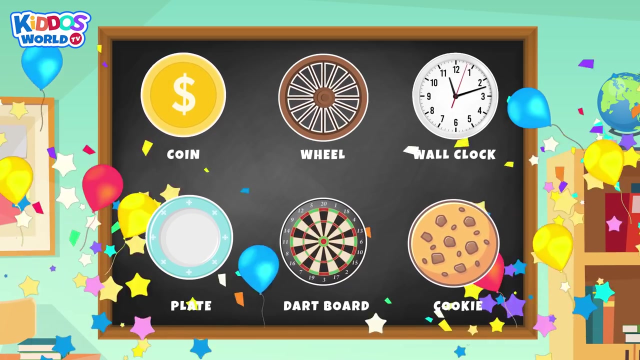 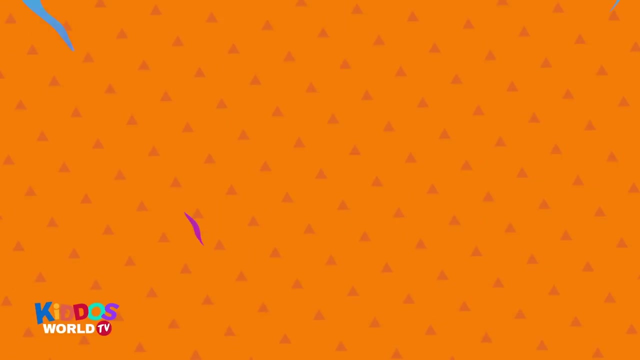 Good job. Circles are also frequently seen around us. Let's identify some of them: Coin, Wheel, Wall, clock, Plate, Dart board, Cookie. Well done, Let's move on to our next shape: Triangle. A triangle has three sides And is formed when three straight lines meet. 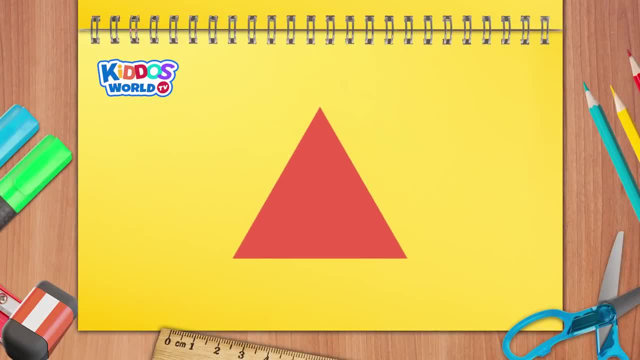 Now let's practice and draw the triangle with me From the top. draw a diagonal line to the left And another diagonal line to the right. To finish, draw a straight line at the bottom. Amazing work. Now let's identify things that are triangular in shape. 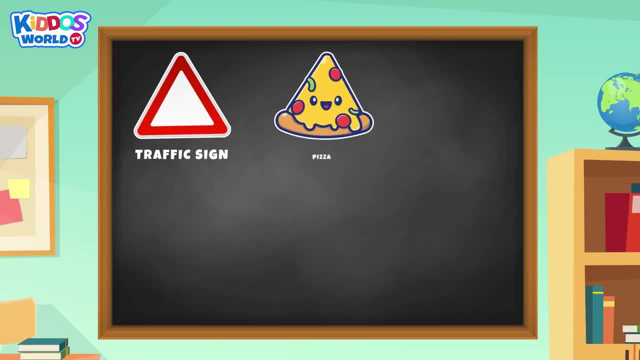 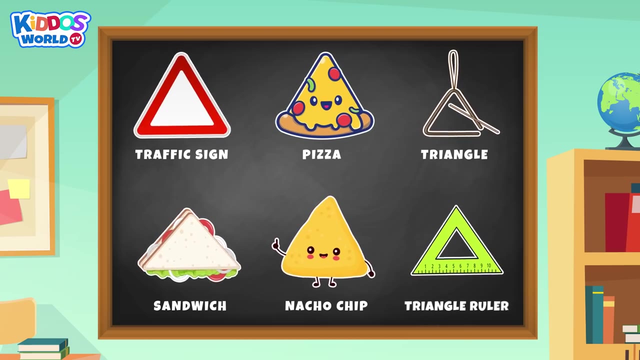 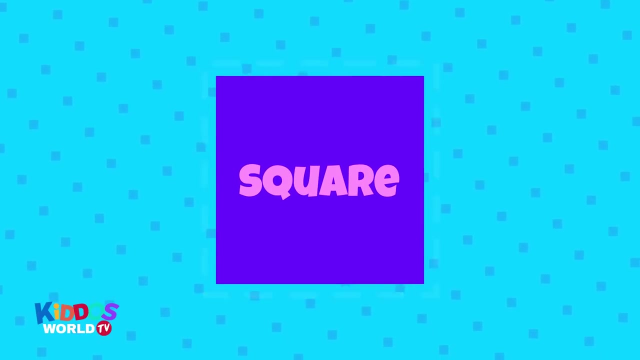 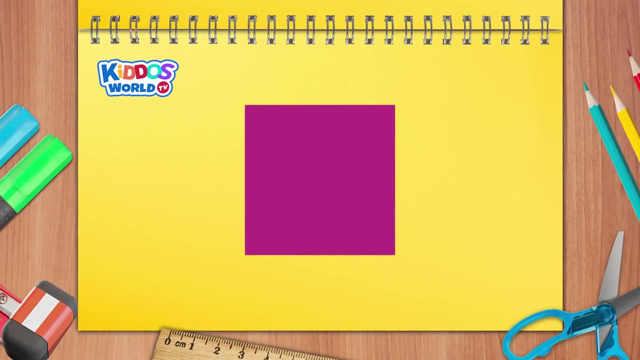 Traffic sign: Pizza Triangle, Sandwich, Nacho chip Triangle ruler. Yay, Our next shape is… A square. Yes, A square is a shape with four sides of equal length. Now let's make a square From the top, draw a straight line and pull down. 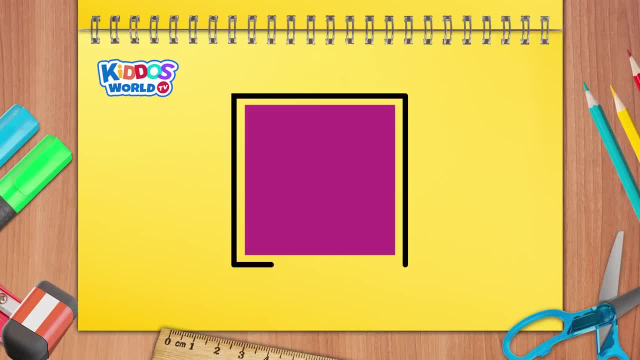 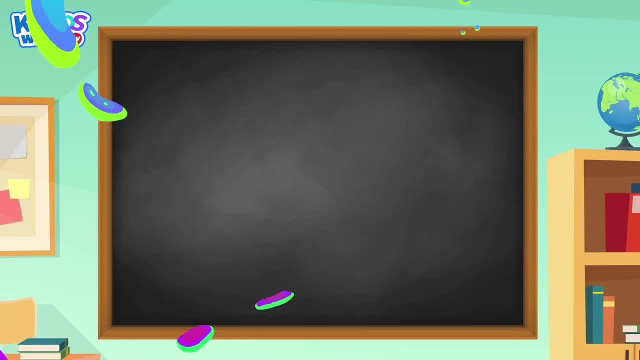 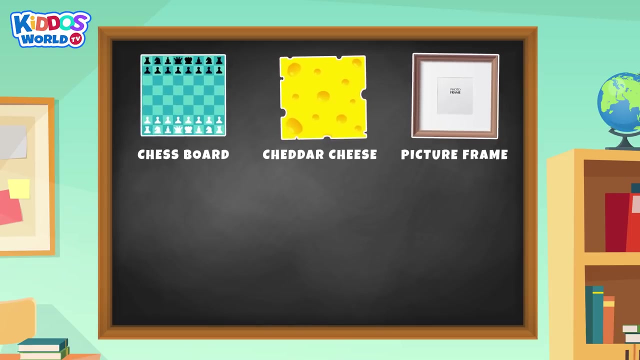 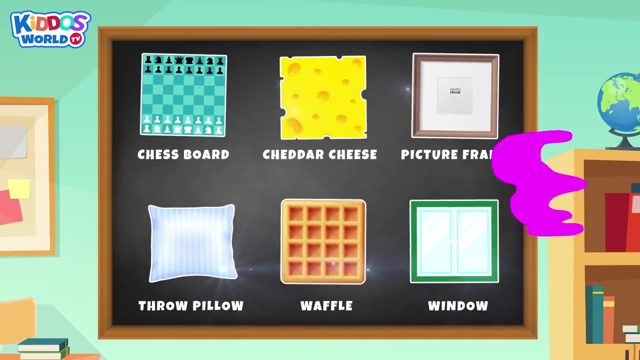 Now pull down on the other side To finish. draw a straight line at the bottom. You're doing great. Here are examples of things that are: square: Chess board, Cheddar cheese, Picture frame, Throw pillow, Waffle Window. Our next shape is an interesting one. 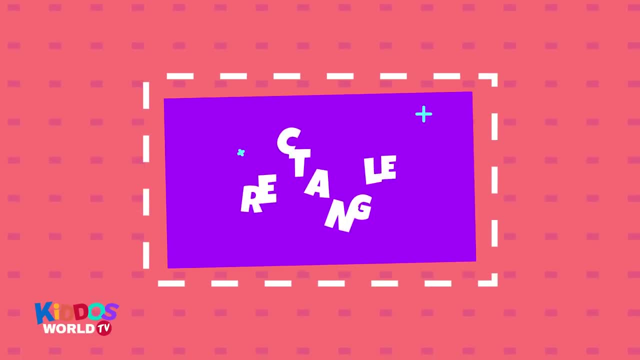 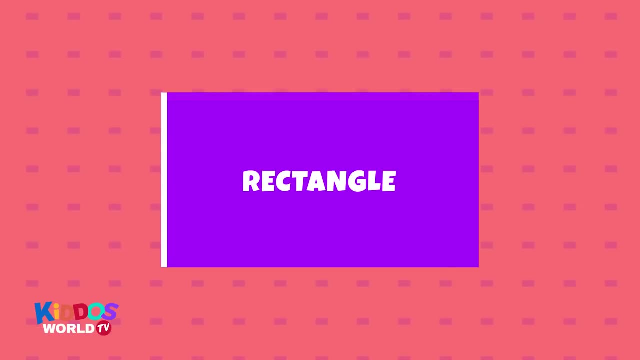 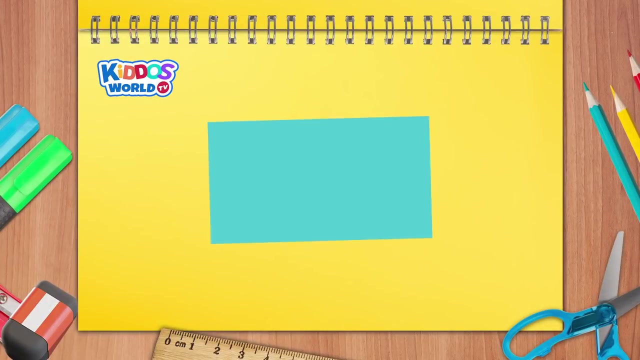 A rectangle. A rectangle, just like the square, also has four sides, But with two sides being longer than the other two. Now let's practice and draw the rectangle. Draw a longer straight line across the top, From the top, pull down and pull down on the other side. 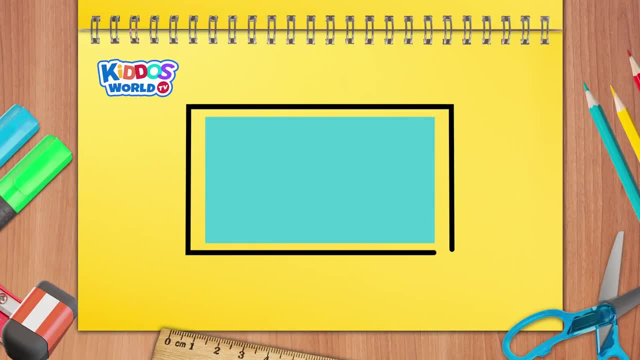 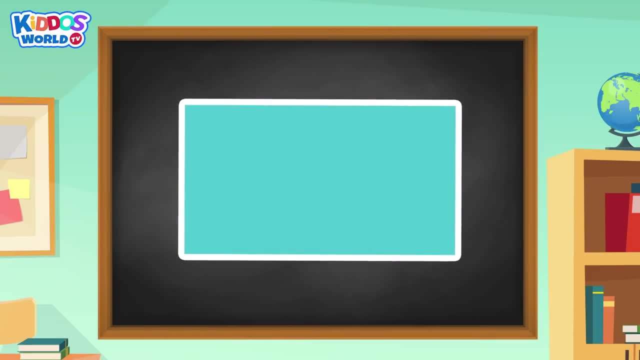 Then draw another straight line across the back From the top, pull down and pull down on the other side. Then draw another straight line across the bottom. You're really good at this. Now let's identify things that are also rectangular in shape. 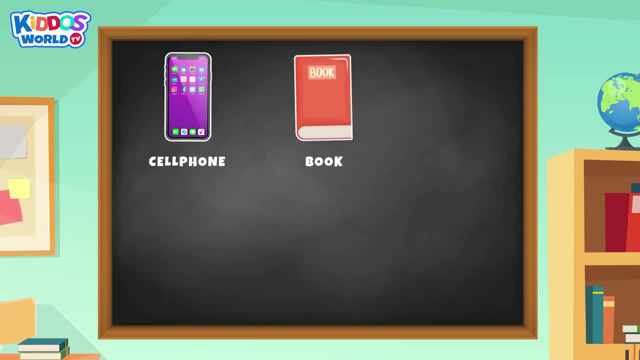 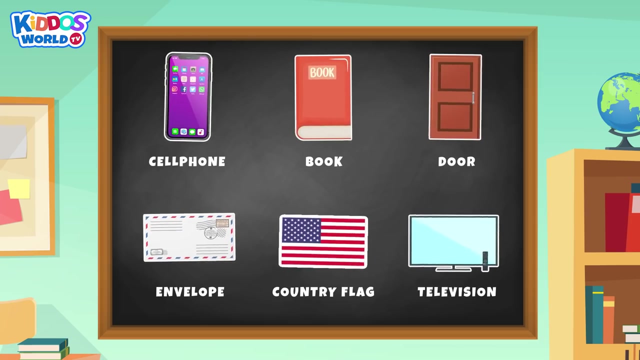 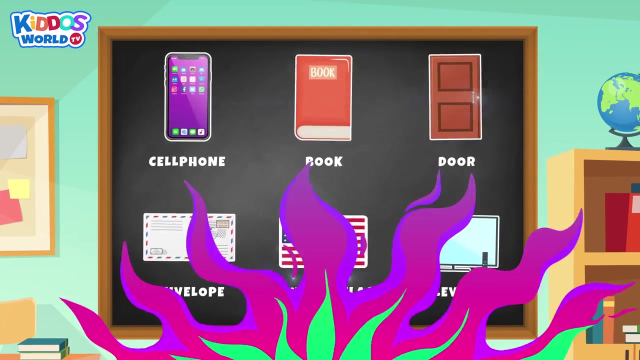 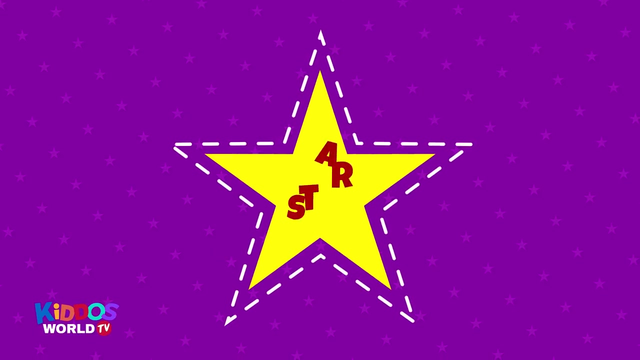 Cell phone, Book Door, Envelope Country flag Television. This next shape is a special one. We see it shining every night: A star. A star is a shape with five sides. It's like putting five triangles and a pentagon all together. Now let's practice making one. 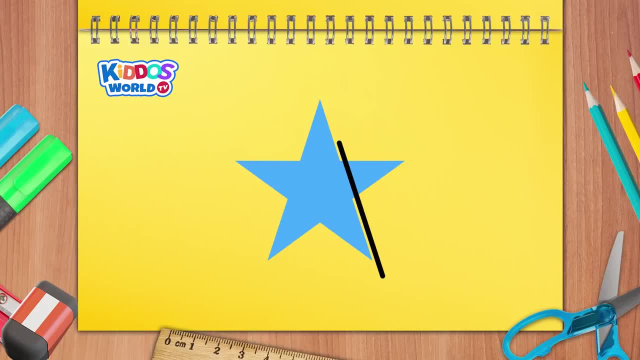 From below, draw a diagonal line going up And draw a diagonal line down to the left. Then draw another diagonal line going up, Now a straight line across. To finish, draw a diagonal line heading to the bottom left and close. Wow, Amazing work. 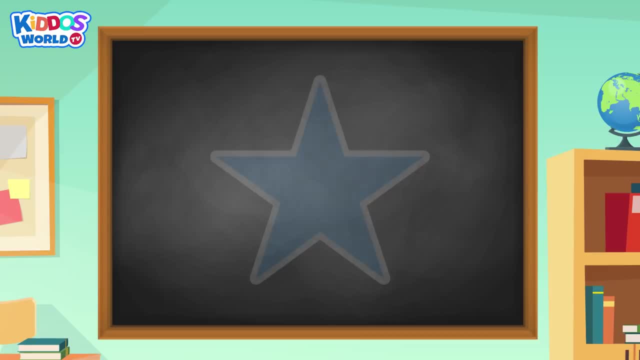 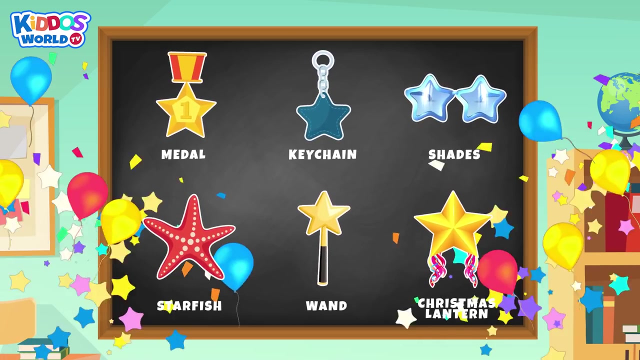 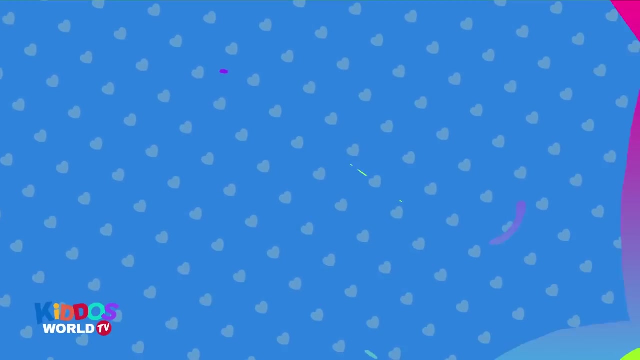 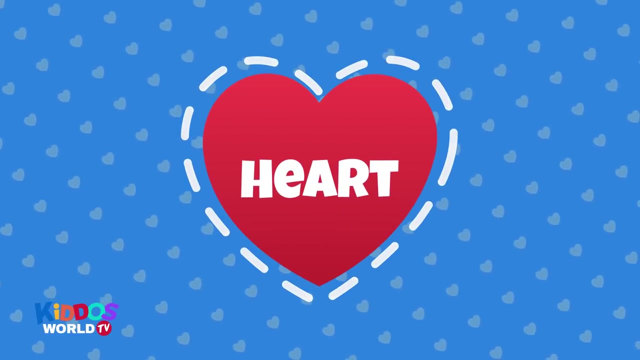 Here are some star-shaped items around you, Left items around us: Metal Keychain, Shades, Starfish Wand, Christmas lantern. Our next shape is a lovely one. You guessed that right: A heart. A heart is a shape made out of two curves. It is also a symbol of love. 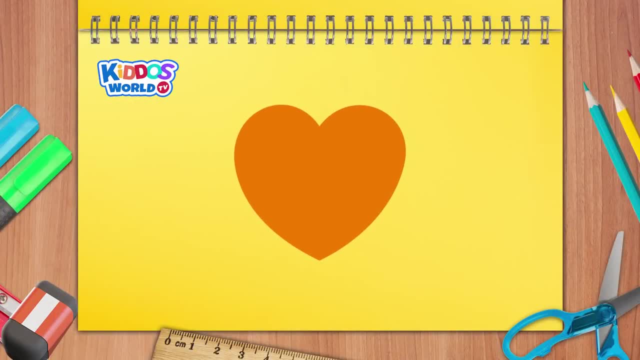 Now let's learn how to draw a heart From the top. draw a curve to the left, going down at the bottom center. From the bottom, draw another backwards curve to the right, going up to the top center, and close Ow. 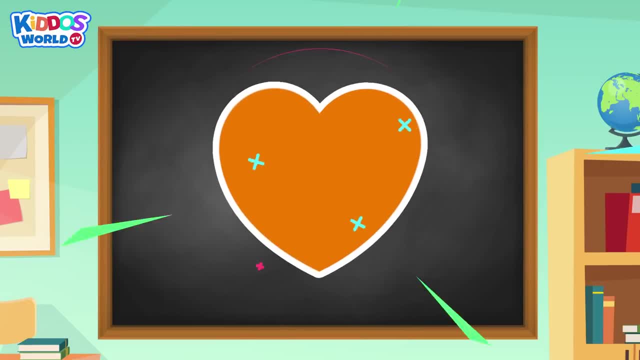 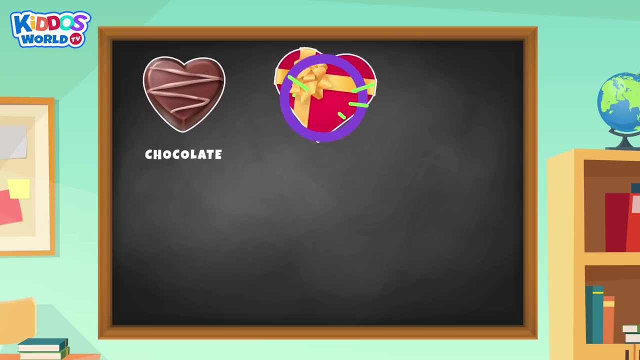 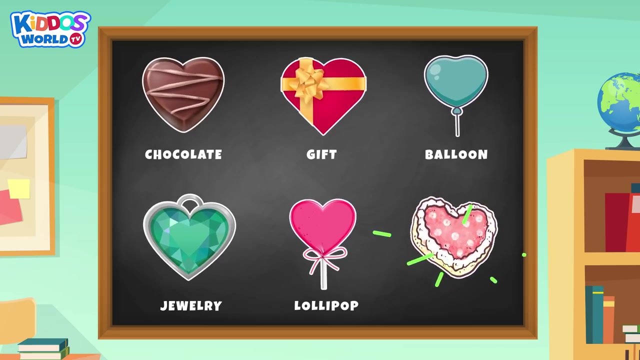 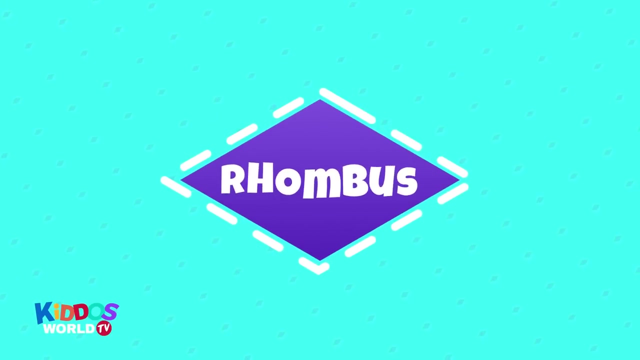 Oh, that's lovely. Let's identify these heart shaped items. Let's see the heart shaped items. Chocolate, Chocolate, Gift, Gift Balloon, Balloon, Balloon, Balloon, Balloon, Jewelry, Jewelry, Jewelry, Jewelry, Jewelry, Jewelry, Lollipop, Lollipop, Lollipop Cake, Cake. for sure you will like this next shape, the rhombus. a rhombus is a shape that resembles. 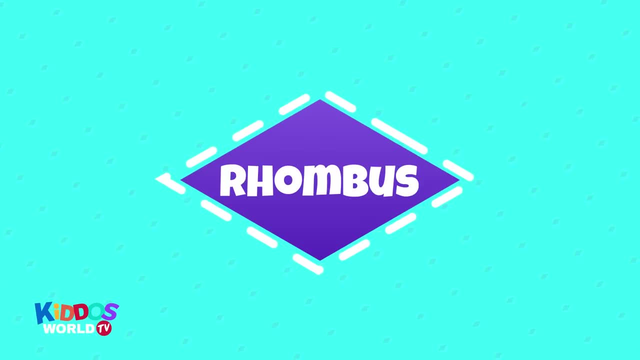 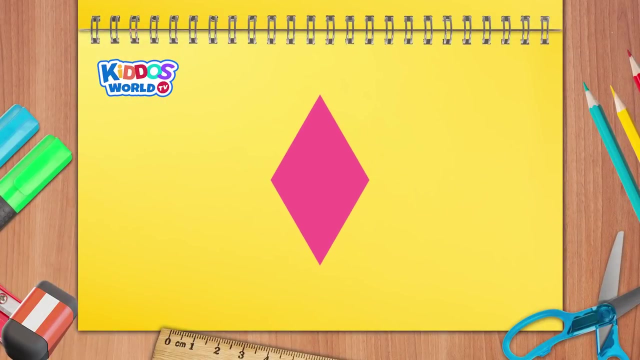 a diamond. unlike the square, a rhombus is quadrilateral in shape, in which opposite sides are parallel and opposite angles are equal. now let's figure out how to draw a rhombus. from the top, draw a diagonal line to the right, going down to the middle. then draw a diagonal line to 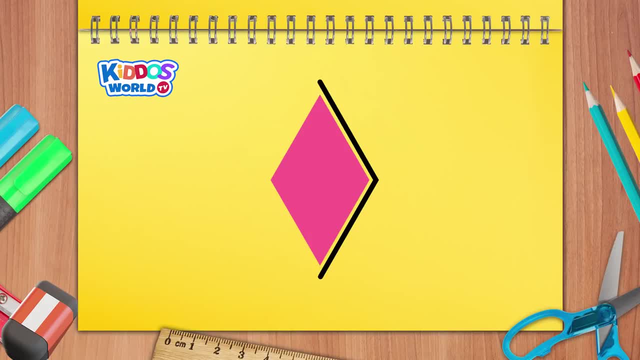 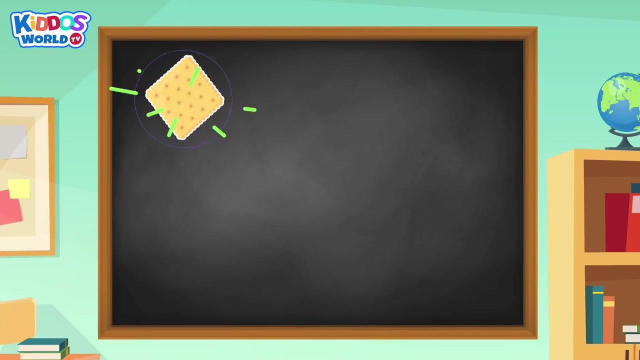 the left going down at the bottom center. from the bottom center, draw a slant line to the left up to the middle and, to finish, another diagonal line to the right, going up to the center top and close. very good, what are real-life items that are shaped just like a rhombus? here are some examples: crackers. 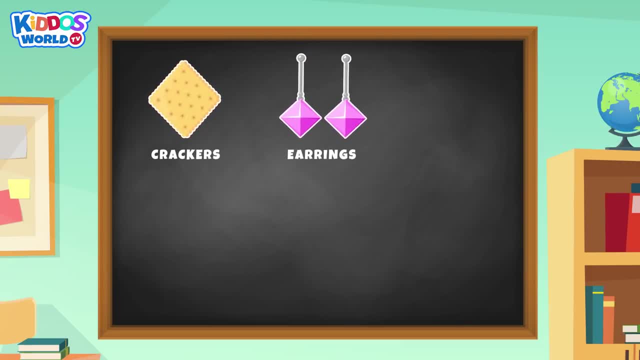 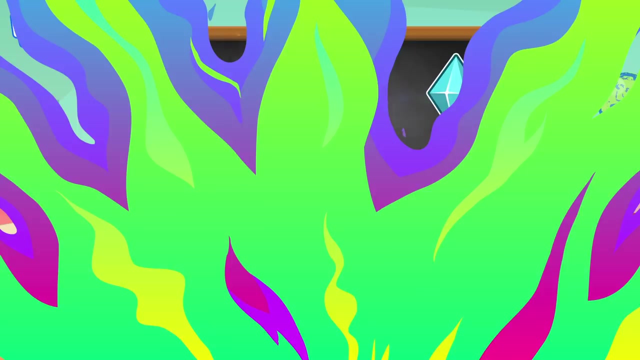 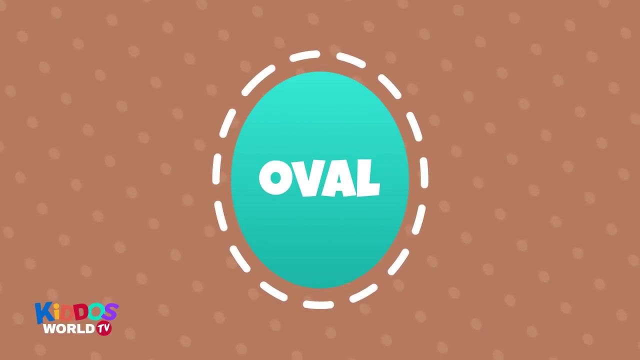 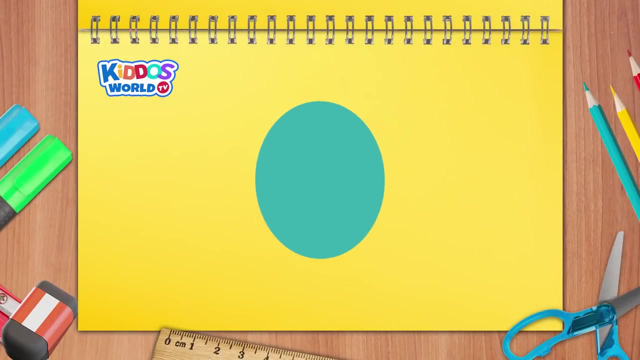 earrings, diamond, kite, signboard tile. we're down to our last shape: an oval. an oval is a closed, curved shape with no straight lines. it also resembles the outline of an egg. now let's practice how to draw an oval from the top center. draw a slightly longer curved line to the left, all the way down to the bottom.